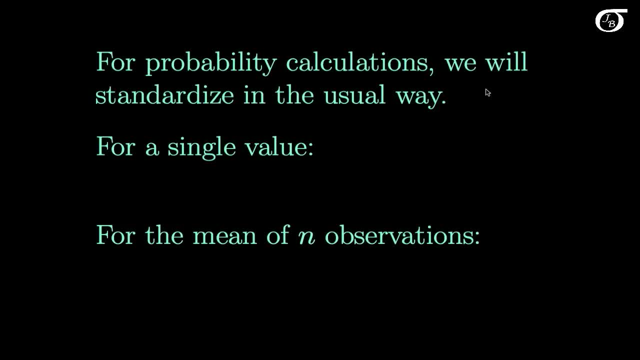 So for a single value, if we have some random variable- x say, that's normally distributed, then when we are standardizing for a single value, we say that z is equal to x minus its mean over its standard deviation, and we've done that previously. 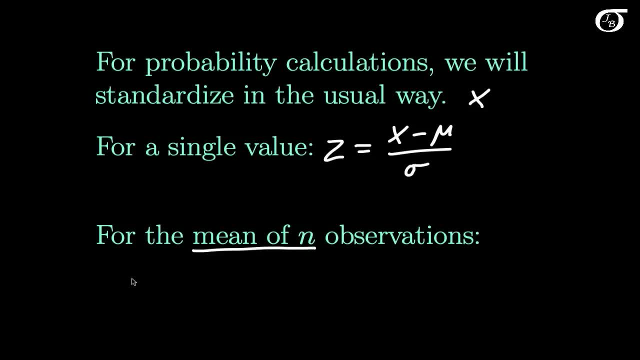 But for the mean of n observations: when we're standardizing, we would do a similar thing. z is equal to the sample mean, x-bar, minus its mean, which just happens to be mu over the standard deviation of x-bar, And this is simply x-bar minus mu over sigma, divided by the square root of n. 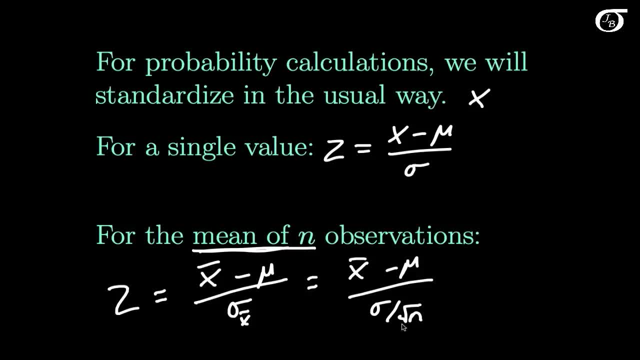 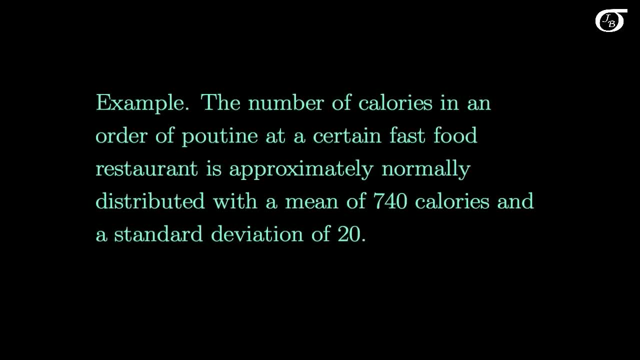 So if we're talking about the mean of n observations, we need to remember to include the square root of n down here. Let's look at an example: The number of calories in an order of poutine at a certain factor. a fast food restaurant is approximately normally distributed. 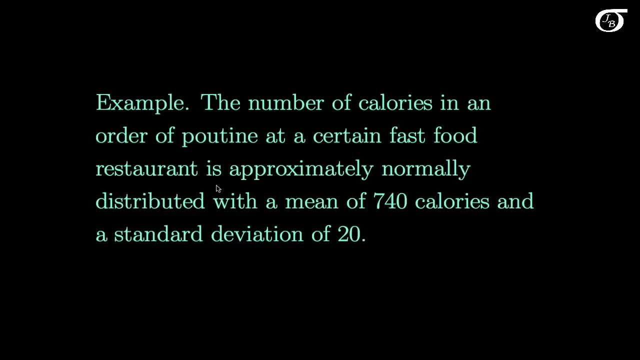 with a mean of 740 calories and a standard deviation of 20.. If you're unfamiliar with poutine, it is french fries, cheese curds and a gravy. Very tasty but also not so good for you At a certain fast food restaurant around here. 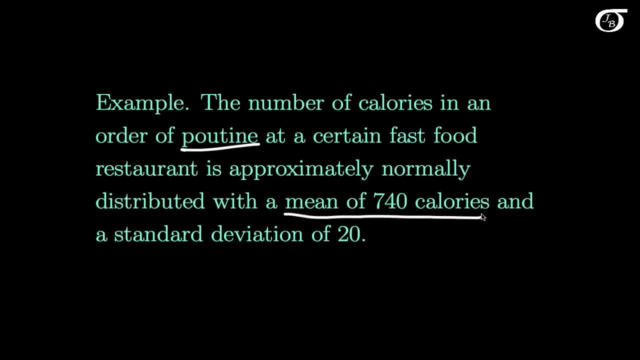 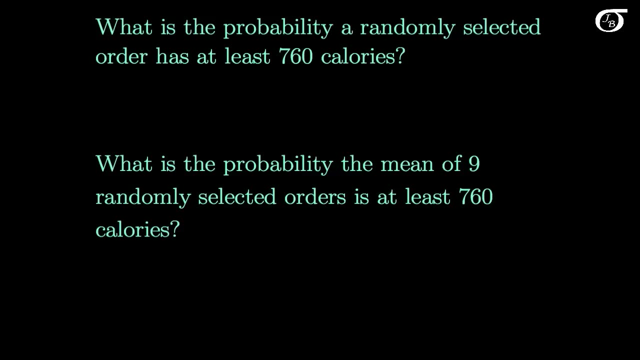 it has a mean calorie content of approximately 740 calories and we're going to say it's normally distributed with a standard deviation of 20 calories. And we're going to do a couple of probability calculations. What is the probability? a randomly selected order has at least 760 calories. 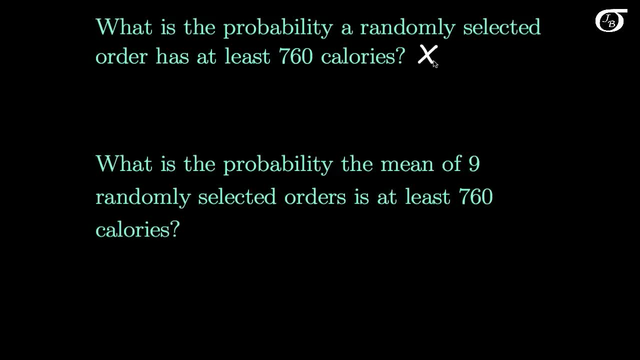 Well, if we let the random variable x represent the number of calories in a randomly selected order of poutine, then x is approximately normally distributed, with a mean of 740 and a standard deviation of 20.. And what we want is the probability that x is bigger than or equal to 760.. 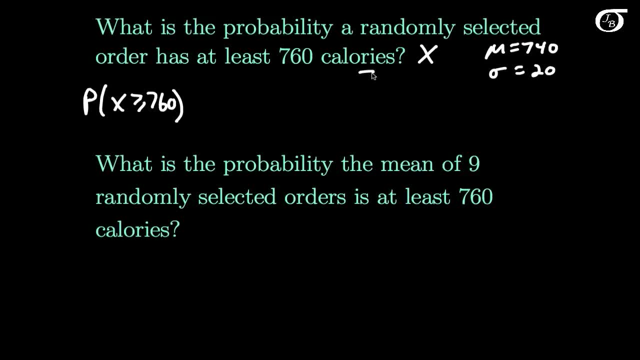 And we're going to standardize this, and we've done this type of thing before. where we standardized it, we said: our z is equal to x minus mu over sigma. So no problem, we can say: this is the probability that z is bigger than or equal to 760 minus 740 over sigma, which is 20.. 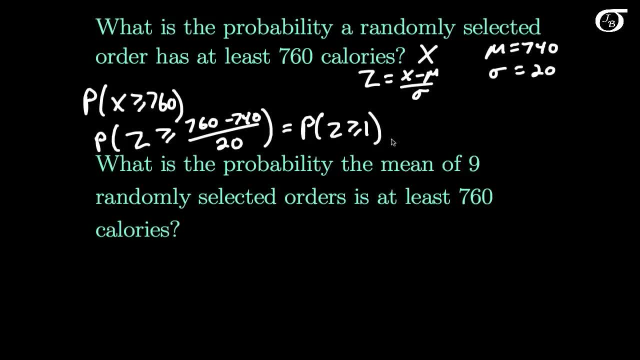 And this is the probability that z is bigger than or equal to 1.. And so if we drew out our standard normal curve- because z has a standard normal distribution- and we went to our normal table or a computer and we moved the area to the right of 1,, 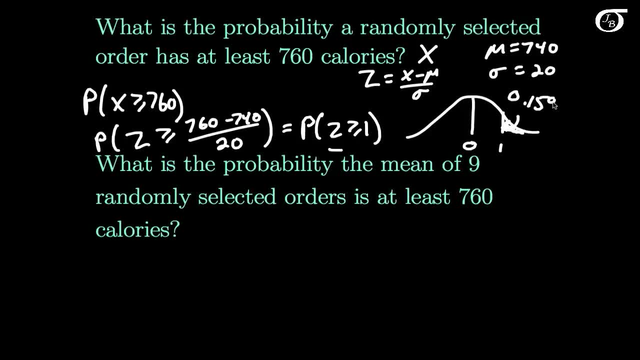 we would see that this is approximately 0.159 to three decimal places. Now a different type of question: what is the probability? the mean of nine randomly selected orders is at least 760 calories. This is fundamentally different because we're talking about the mean of nine of these orders. 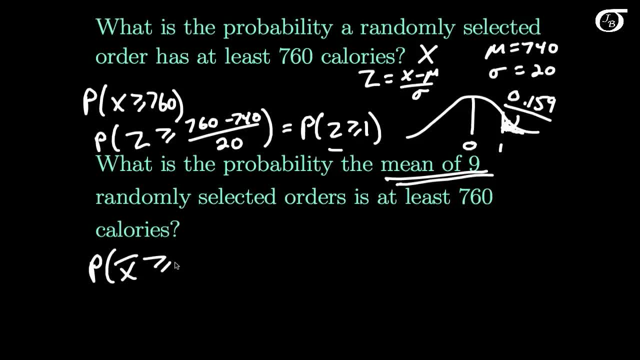 So we want to know the probability that x bar is bigger than or equal to 760.. And we're going to do a very similar test, similar thing to what we did up top. We have to remember that our z is equal to x bar minus mu over sigma. 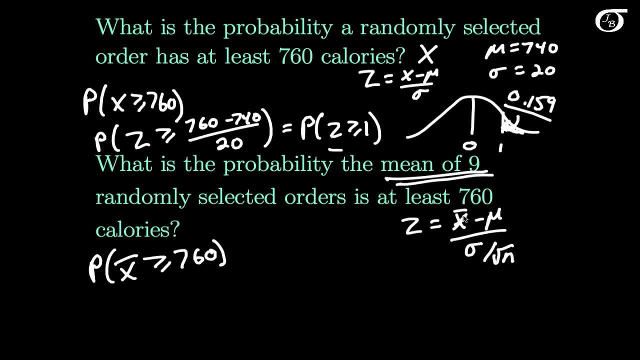 divided by the square root of n, because we're talking about x bar here and not a single observation. so when we standardized here, we say probability, that z is bigger than or equal to 760 minus 740 over 20 divided by the square root of 9.. 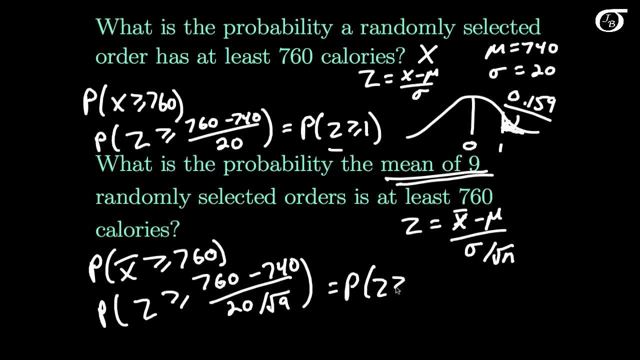 This is the probability. Z is bigger than or equal to 3, where Z has a standard, normal distribution. So we draw this out. we have 0 here, we have 3 out here in this right tail, and we're looking for this area. 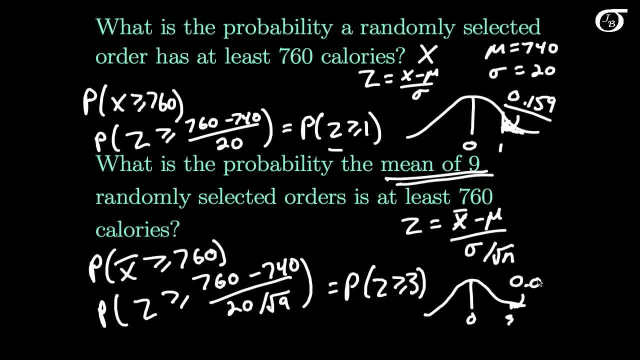 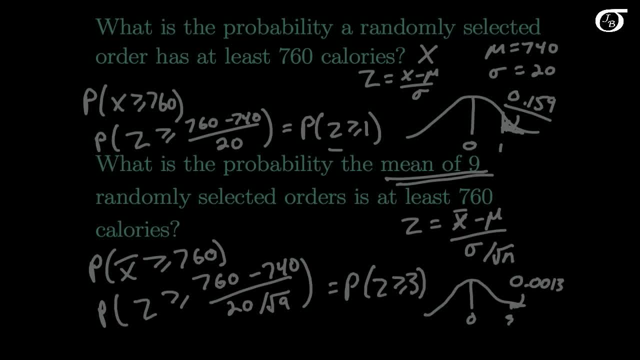 This turns out to be approximately 0.0013. if you put that into a computer or you use your standard normal table to find that area. Now, visually here's what's happening. The solid line is representing the distribution of a single poutine. 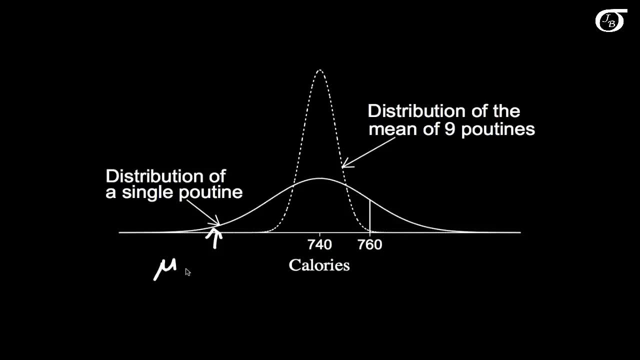 This was approximately normally distributed, with a mean of 740 and a standard deviation of 20.. What we found in the first question on the last page was this area, the area to the right of 760 under this distribution, But when we were talking about the mean, of 9 poutines. 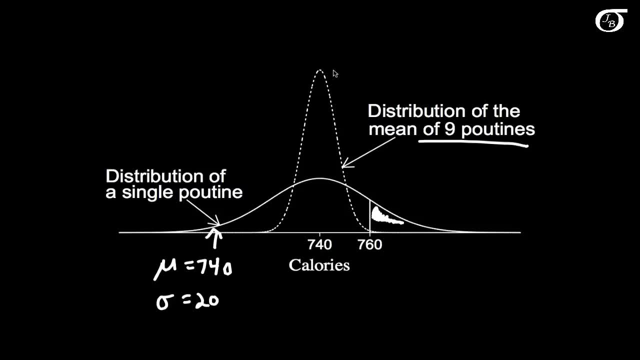 the distribution is a little different. It's very similar. this distribution has a mean of 740, so the same mean as that of a single observation. but the standard deviation of the sampling distribution of X bar was sigma over the square root of n. 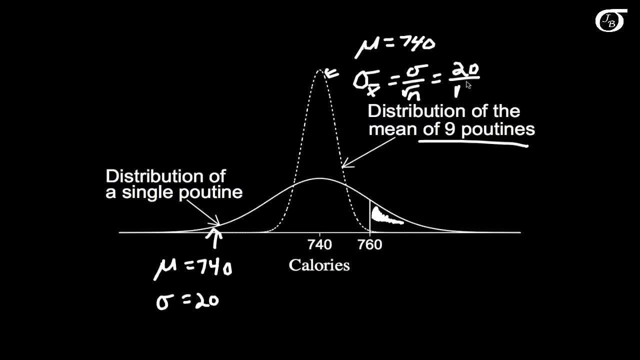 And that was 20 over the square root of 9, which is simply 20 over 3.. So the standard deviation of this distribution is less than the standard deviation for a single value, and we can see that because it has this higher peak.